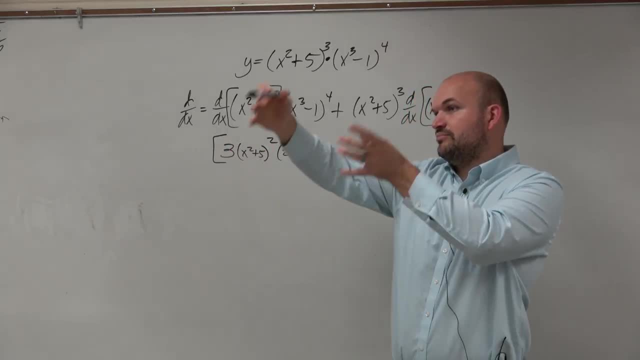 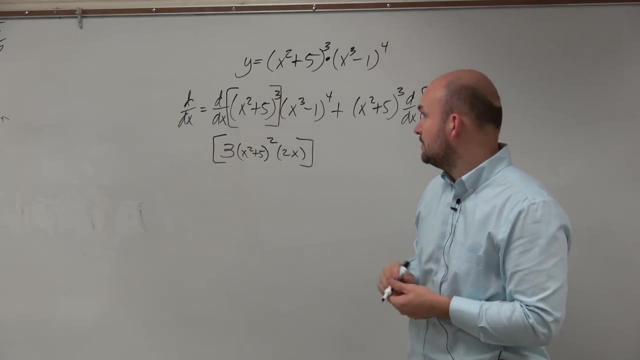 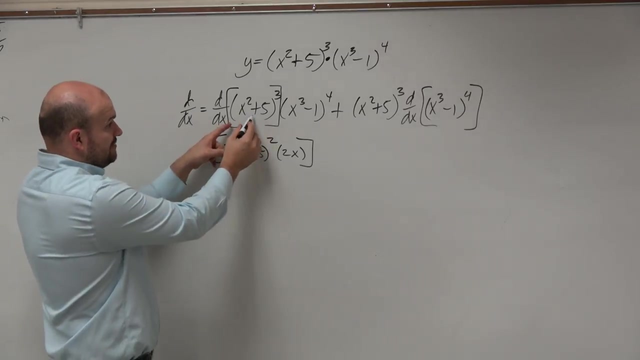 one. And remember you take the derivative of the parent, plug in the child, multiply by the derivative of the child. So the derivative of x squared plus five is just two x. Right, Okay, Now, Yes, Huh, Yeah, yeah, All I did was here to 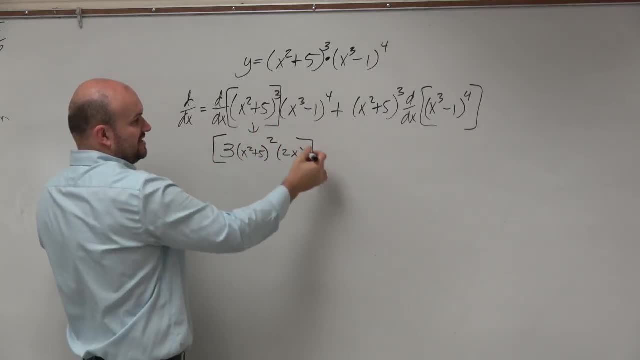 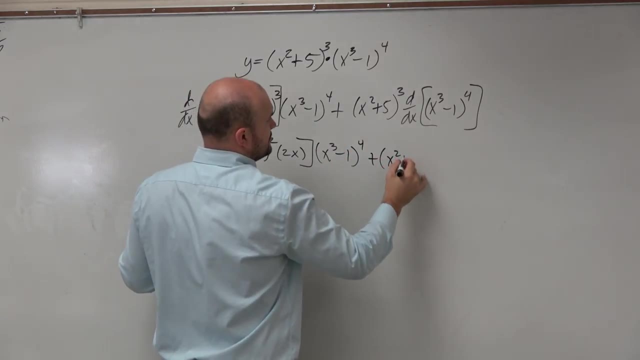 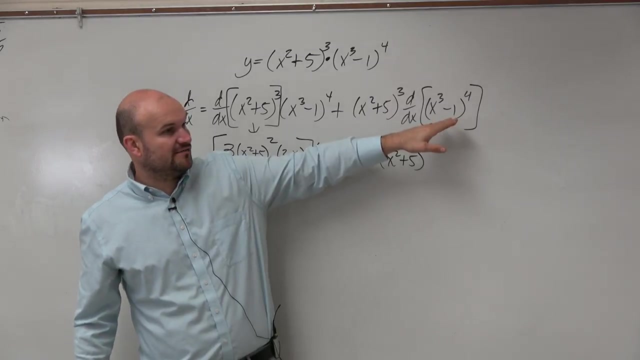 here, I still have all this to go. So now I do this, which is just the same: x cubed minus one to the fourth, plus x squared plus five cubed. And now I need to take the derivative here, which is again: what is the parent function? 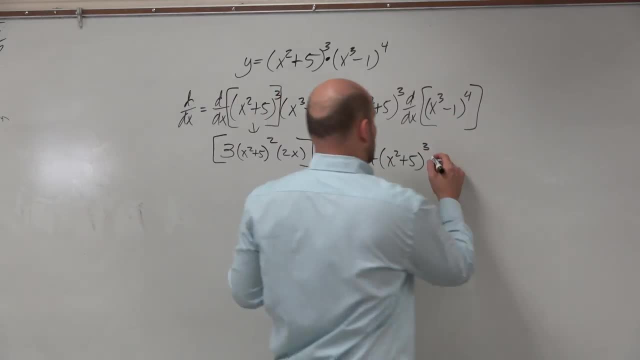 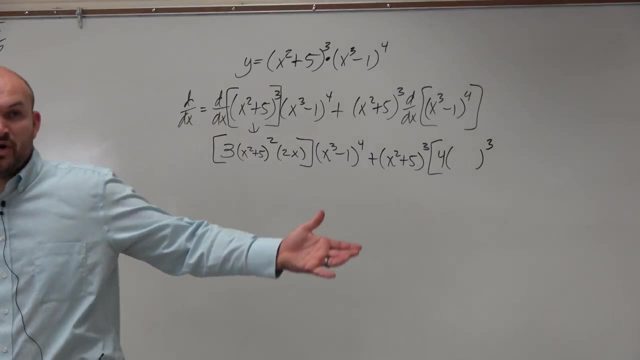 of this one x to the fourth. So if I'm going to do that, I'm going to do four times x to the third. Would everybody agree that's like the derivative of my parent function? Does everybody see that? That's the? 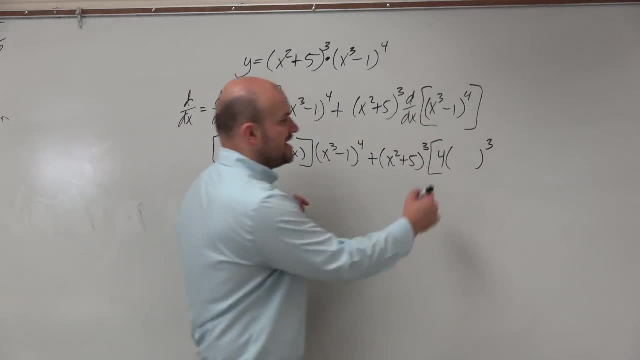 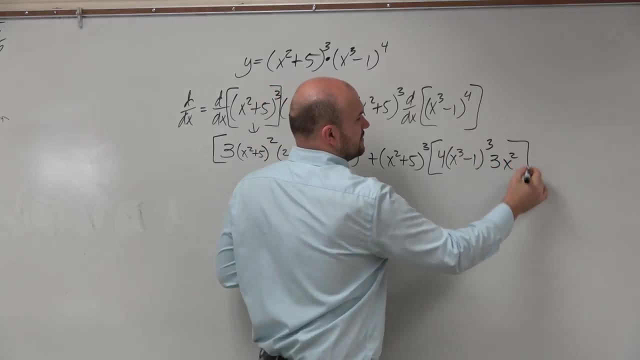 derivative of my parent function. Then I plug in my child function, which is x cubed minus one times the derivative of my child function, which is three x squared. Now we try to look again to see if there's anything that we possibly. 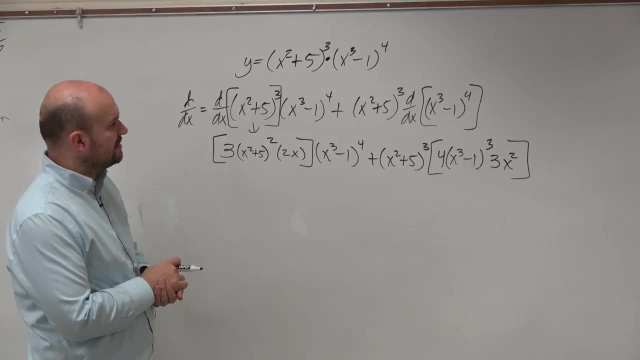 could take out, And there are some things that you know. in reality, guys, these are all just the products, all multiplied by each other, Right? So if you wanted to simplify this, or if you were asked to simplify this, there's a couple things that we could take out. 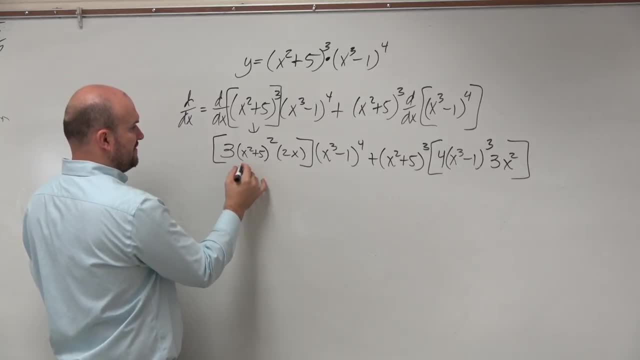 So let's see what they have. Let's see what these two have in common. They have a x squared plus five squared- x squared plus five squared that you could factor out, And we have a, a, three and an x that we could take. 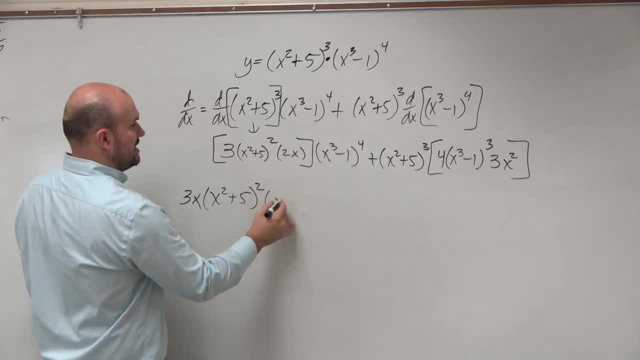 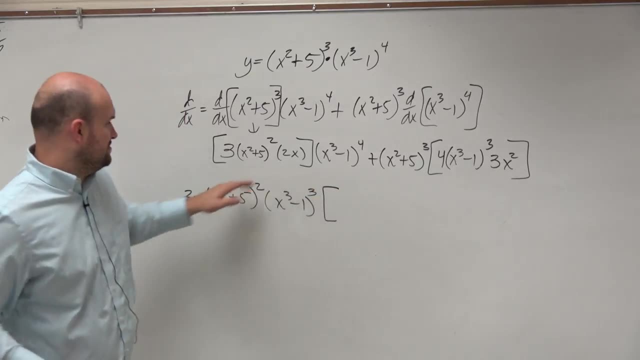 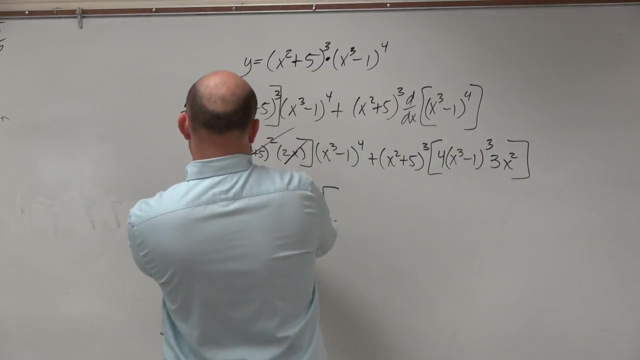 out. And then we have also a x cubed minus one we could, to the third power we could take out. So if we take those both out, the threes would go, the x would go- I'd be- and the two x squared would. 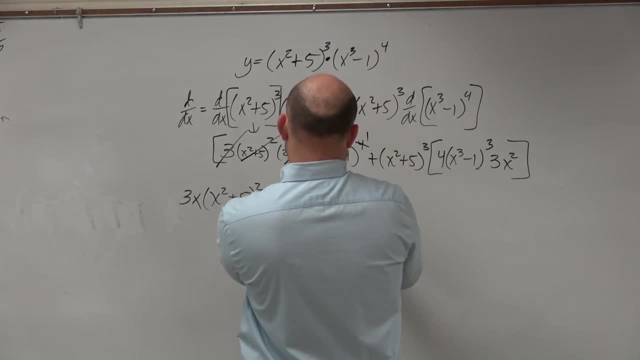 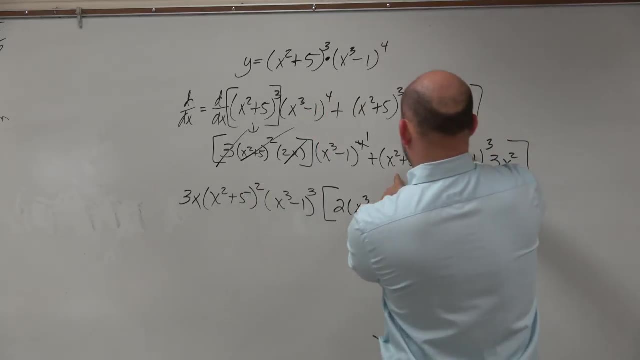 go, and then this would be to a one. So I'd be left with two times x cubed minus one. Then over here, if I pulled out an x squared, that would go to one. The three would divide out The x.